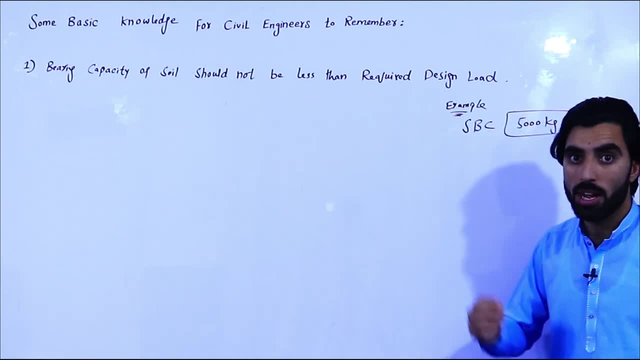 the bearing capacity of sign 5000 kg per meter square and the design load is, for example, if the design load is design load are required load, if that is, guys, 10 000 kg per meter square, so the foundation will be failed because the design load is 10 000 kg per meter square. 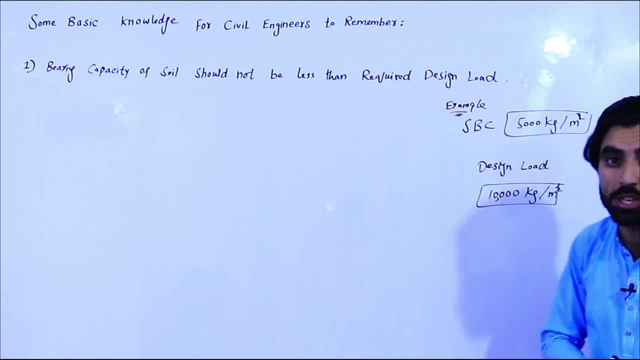 and sbc style. bearing capacity is 5000 kg per meter square. so what do you think about this? so, therefore, bearing capacity of the side should not be less than required design load. so we should put what factor of safety? there should be minimum 1.5 time, okay. how? for example, if the design load 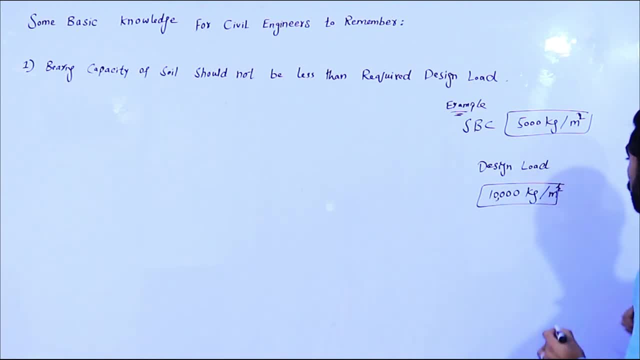 is 10,000 kg per meter square, so the side bearing capacity should be minimum 25,000 kg per meter square. so this should be the bearing capacity of side. if the design load is design structure load is which apply on the side, which transfer to the side. if that is what, 25,000, okay, if that is 10,000 kg per 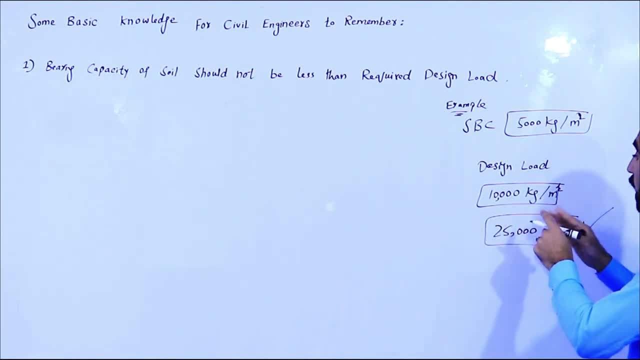 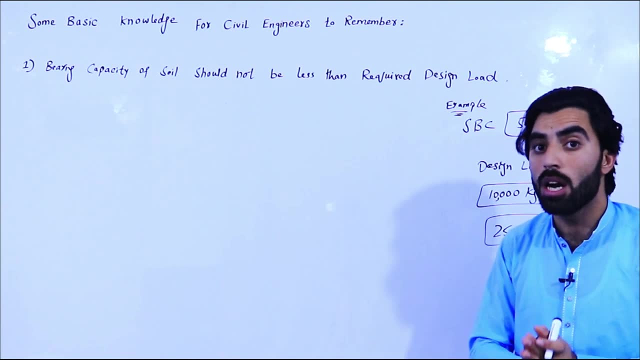 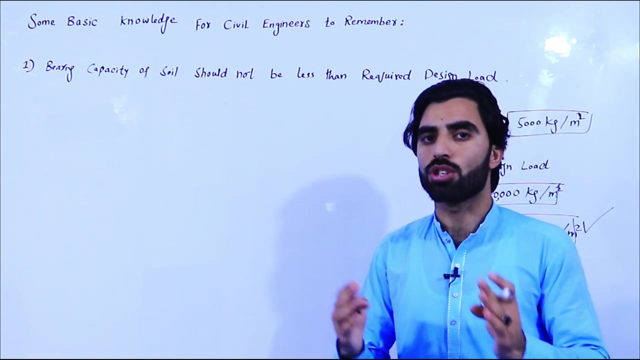 meter square design load, our structure load per meter square and the side bearing capacity should be not less than 25,000 kg per meter square because we should keep the what factor of safety, otherwise you will face the problem. so the bearing capacity of side should not be less than required design load, otherwise you will face the 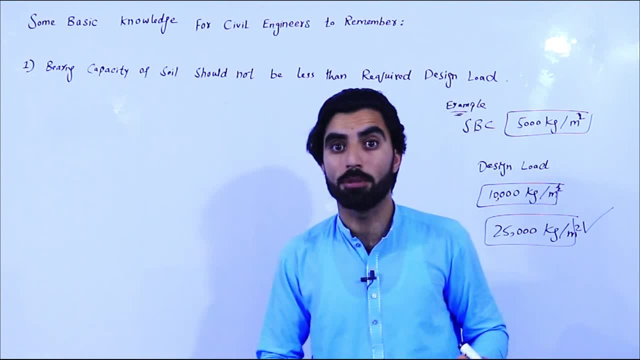 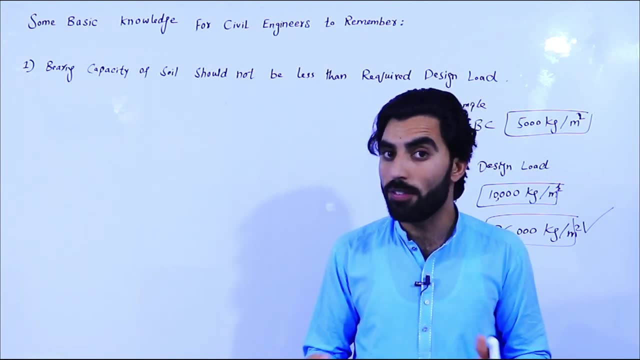 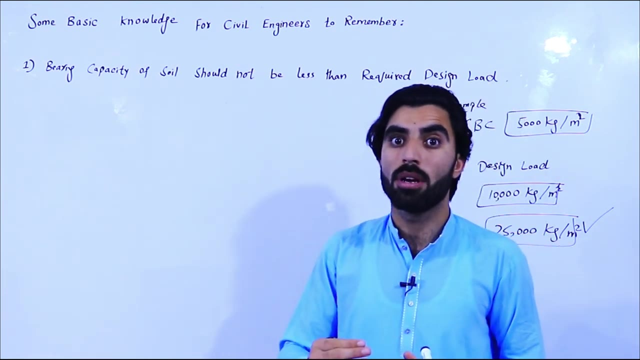 problem. so if the bearing capacity of the cell is 10,000 kg per meter square and the structure load is also 10,000 kg per meter square, so you will face more problems after completion of the design load construction. so therefore the bearing capacity of the side should be maximum. 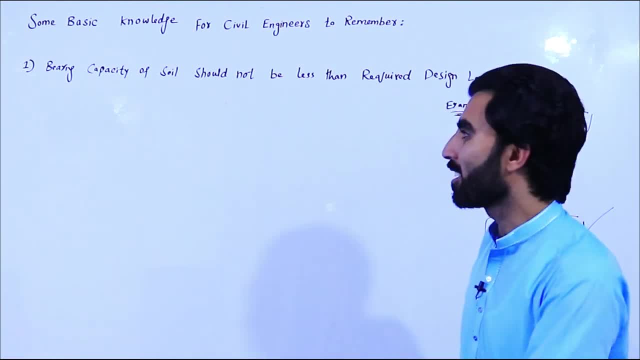 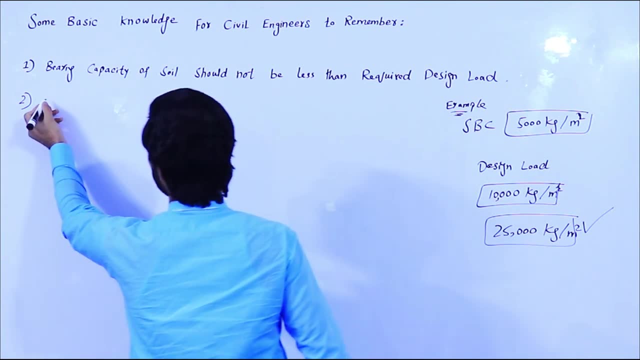 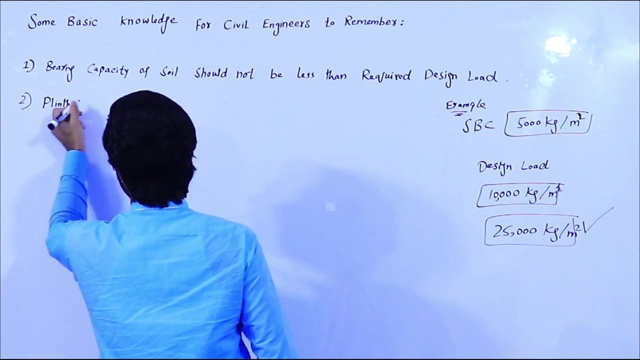 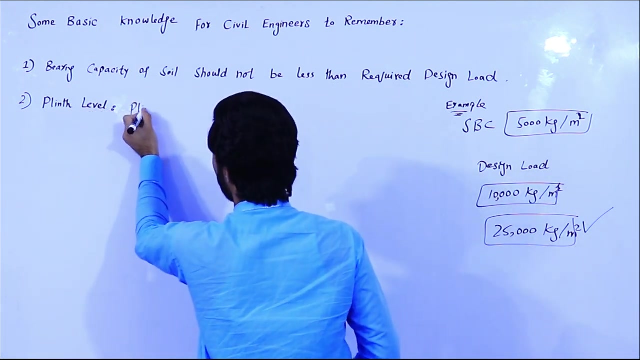 from the design, our structure load right. got it the point or not? this is the main point. second, guys, plinth level of construction. plinth level of house. okay, so the plinth level. remember, guys, that the plinth level of construction should be less than 25,000 kg per meter square. 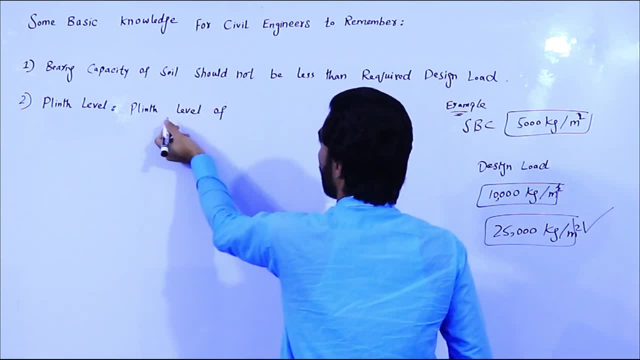 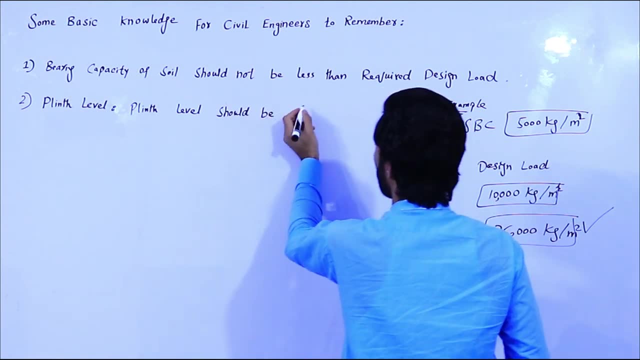 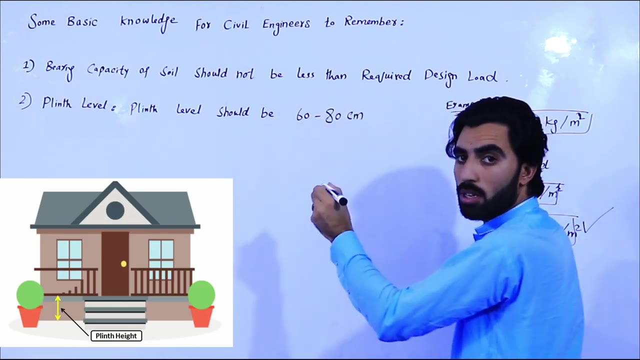 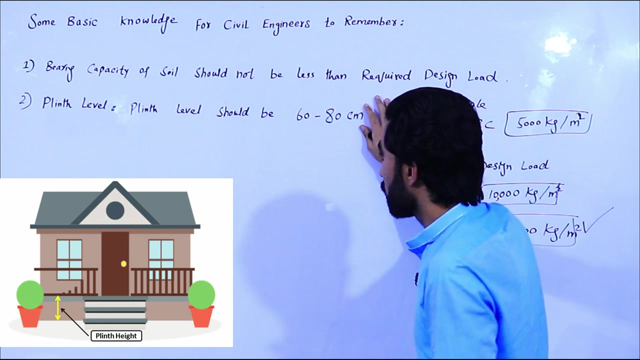 so if the space between VA is 10,000 and 35,000 kg per meter, by saying 50,000 kg per meter. so in case of our structure load, Okay, plinth level of construction: the plinth level should be 60,000 to 80 centimeters. from theild Adrian Maria'll level should be 60,000 to 80 centimeters. from theelet hood sead level should be 60,000 to 80 centimeters. from the imaginarion level se�k ground level should be 60,000. must respect from vec. 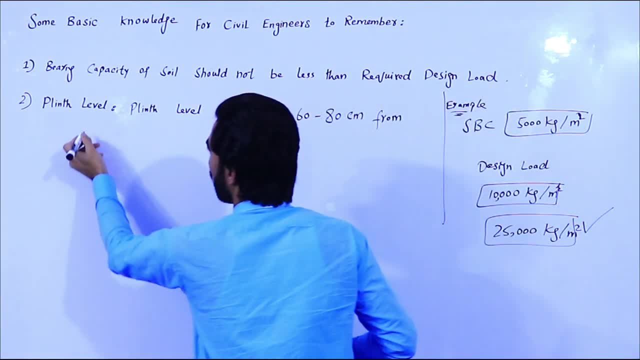 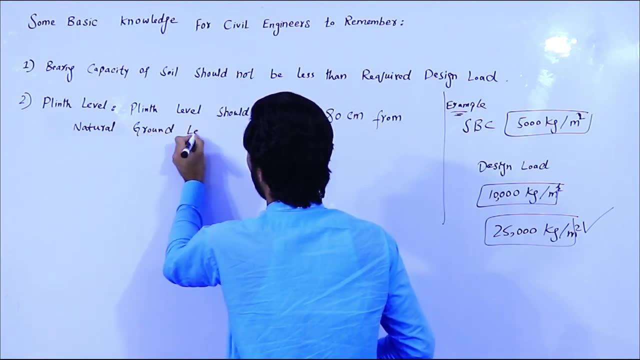 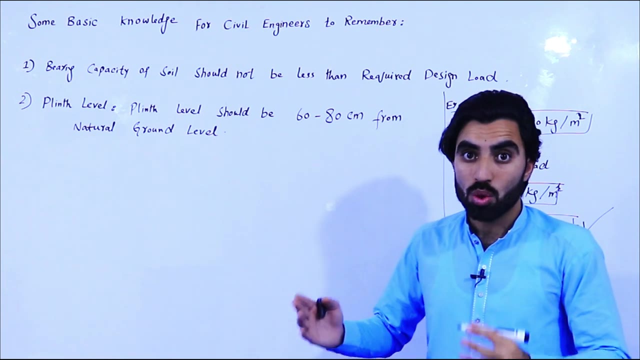 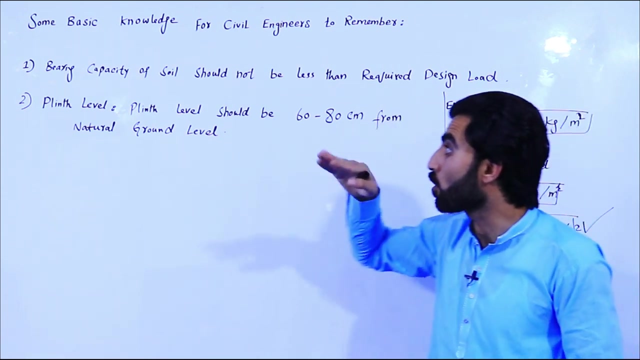 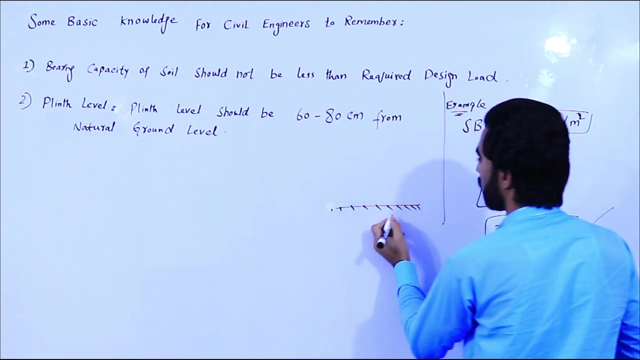 from natural ground level, due to flood, due to rainy water, etc. so, guys, the plant level of house construction should be minimum: 60 to 80 percent from the natural ground level, for example. if you can see, this is the ground level, this is the ground level. so, guys, the plant level of the 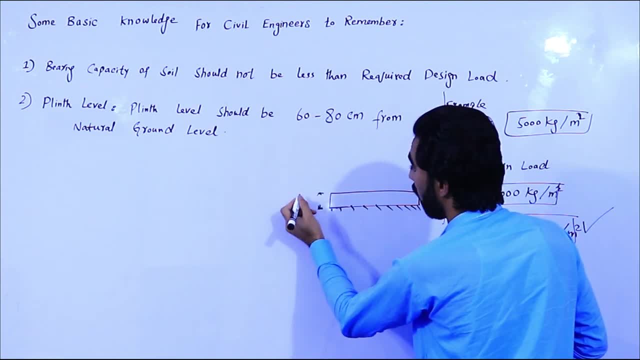 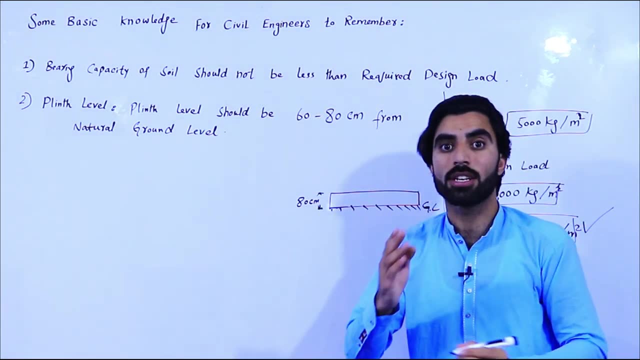 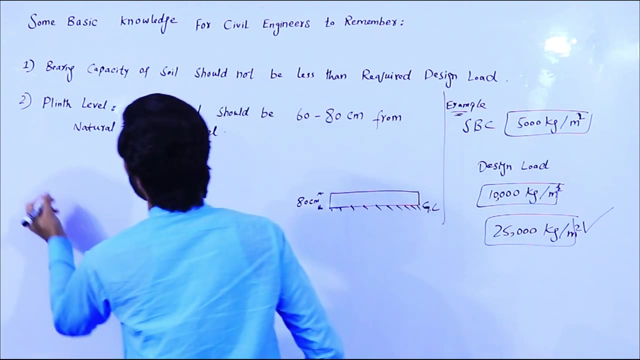 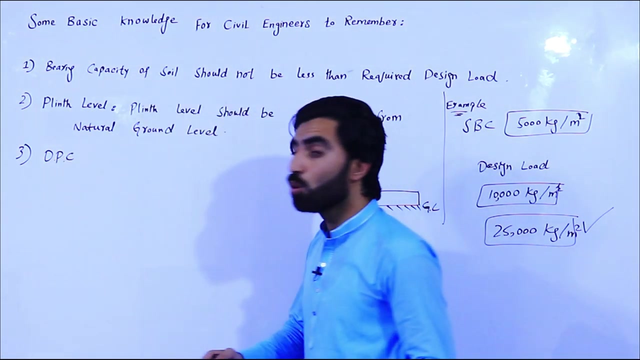 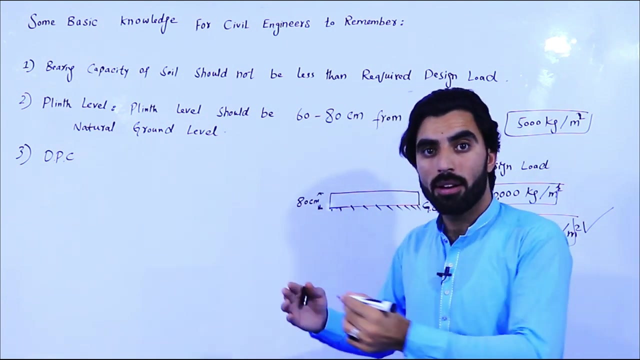 house should be minimum with the height of 60 to 80 centimeter from the ground level, natural nsl, natural ground level, right? so this is also very important. now, guys, the third point is also dpc, dpc, dam proof course, okay, to protect the moisture from the foundation. so, guys, the dpc. 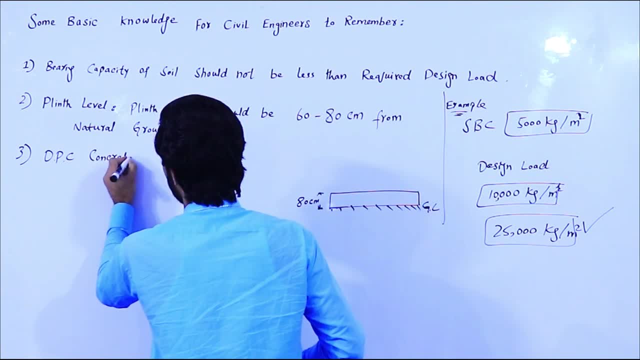 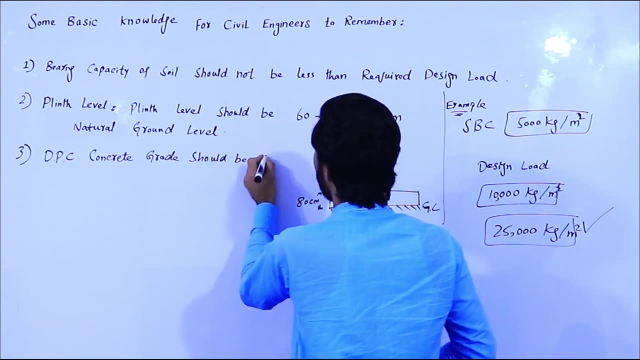 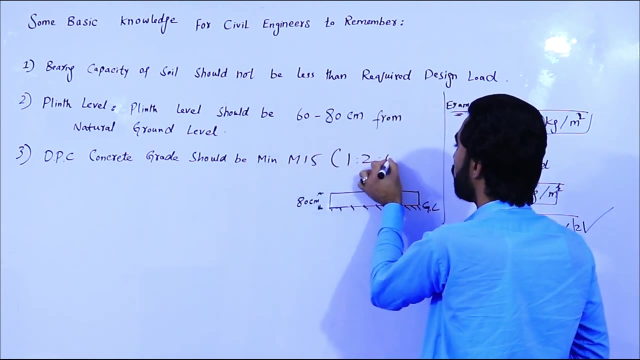 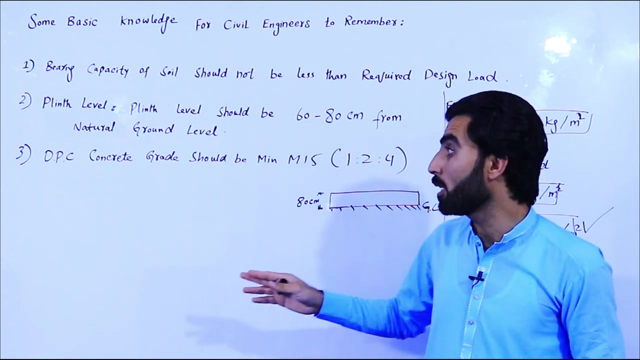 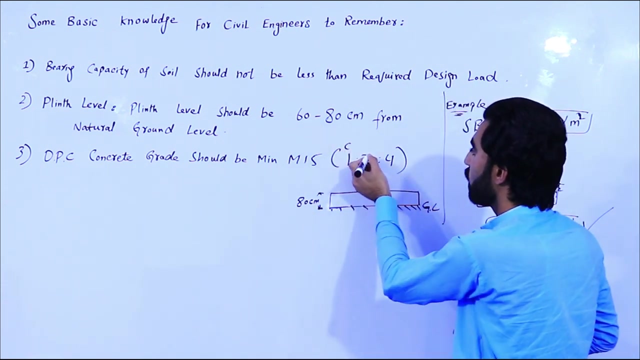 concrete grade should be minimum m 15, which is one to four to make concrete for dpc construction. it should not be less than m15. so we will make a concrete in one to four ratio: one is cement, two is sand and four is aggregate for dpc. with the 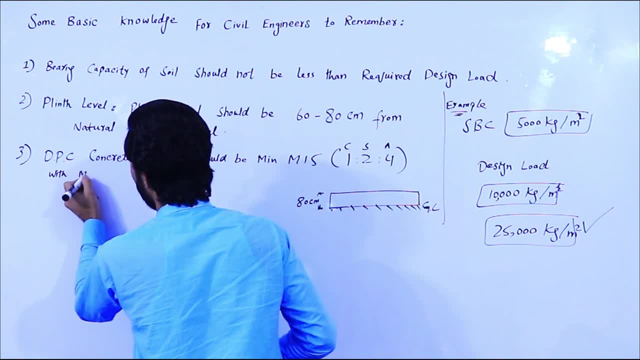 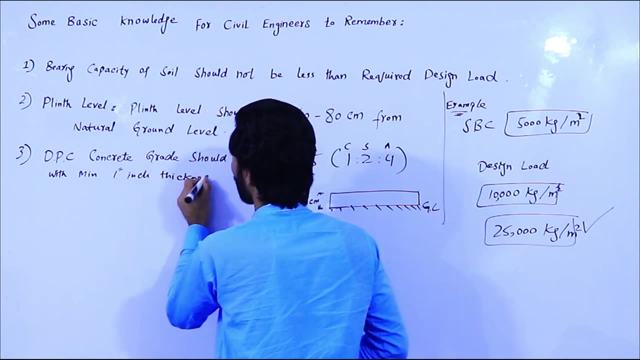 thickness of minimum, with minimum one inch thickness. one inch thickness, minimum one inch thickness. it should be minimum one inch thickness. so, guys, the third point is to make concrete for dpc: shift block that should not be less than one inch, so normally two inch. so, guys, the third point is to make concrete for dpc. 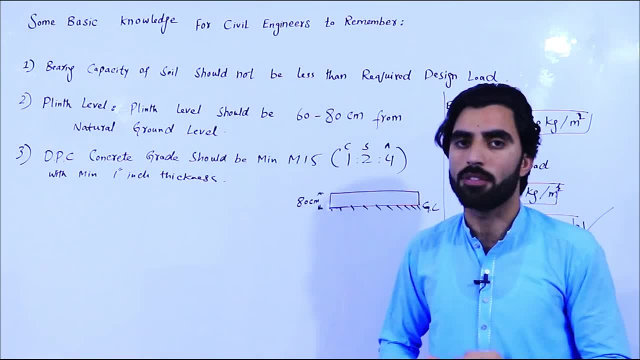 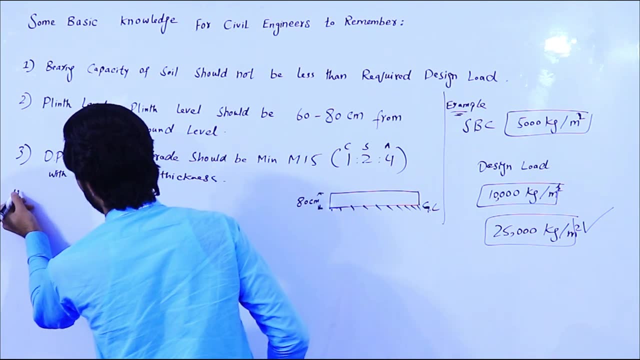 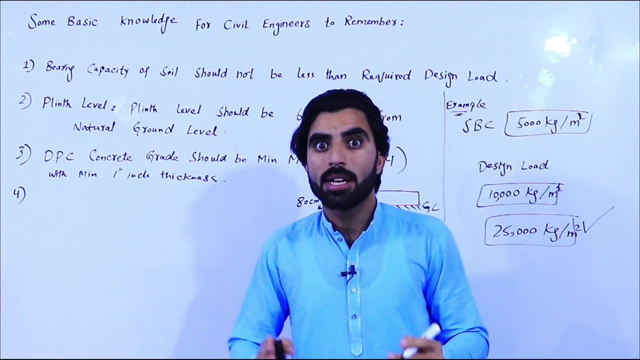 thickness of dd, transportation is quite safe. Okay, this is the other point. now, guys, The other basic point is also, especially for several 1998 millimeters, moment inside: What is the safe distance between two RCC columns? Many students? because, guys, first of all, I will tell you. 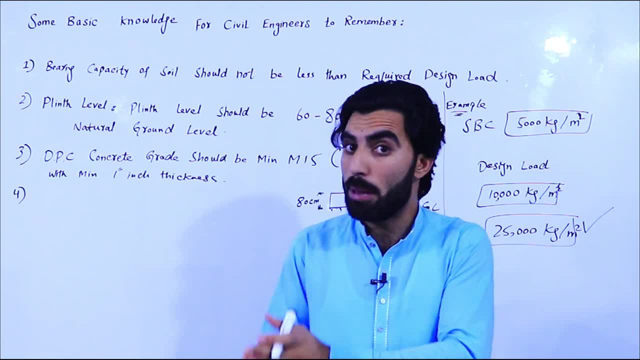 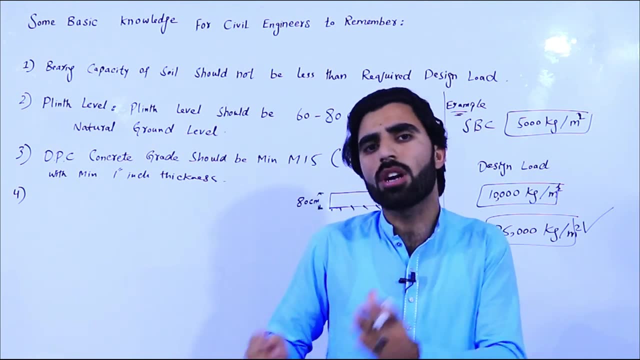 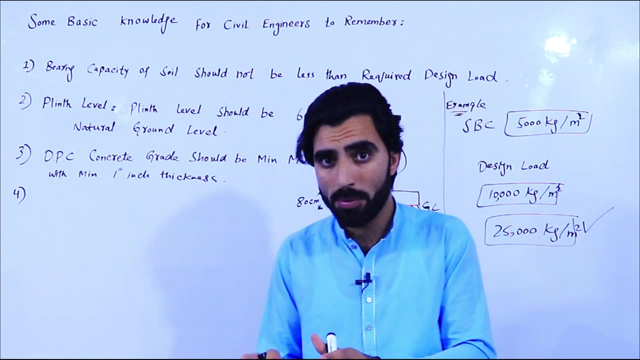 what is the safe distance between two RCC columns? many students because guys for, so for available to you there is. and any limit, any limit in this, in this, because it's depend on the structure load, it's depend on the structure design, etc. so we can't say that the limit is that distance between two rcc column okay, but are the length? 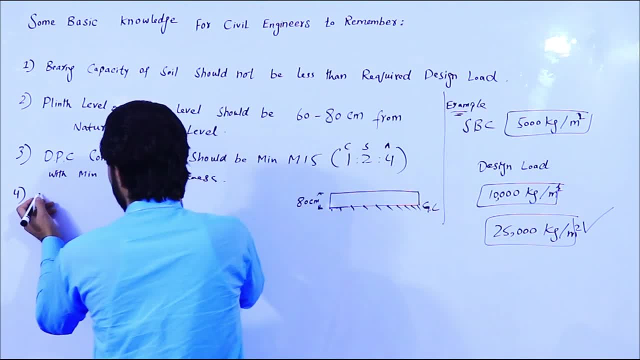 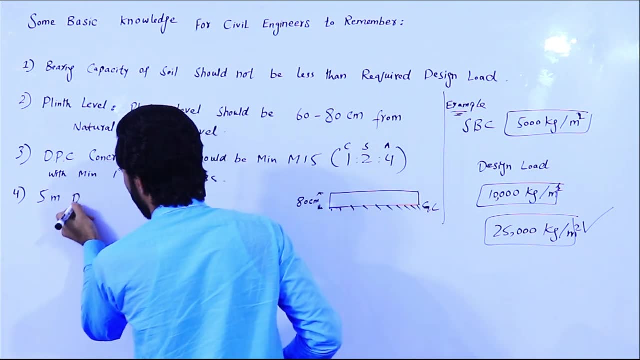 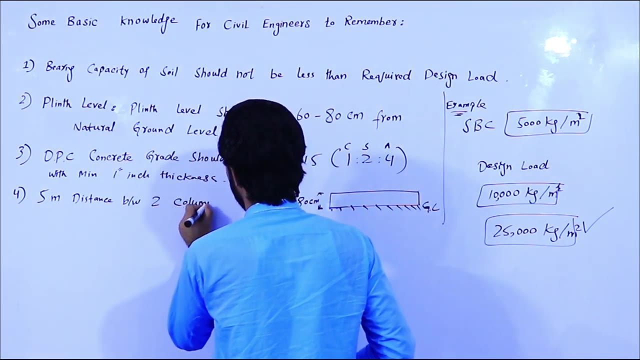 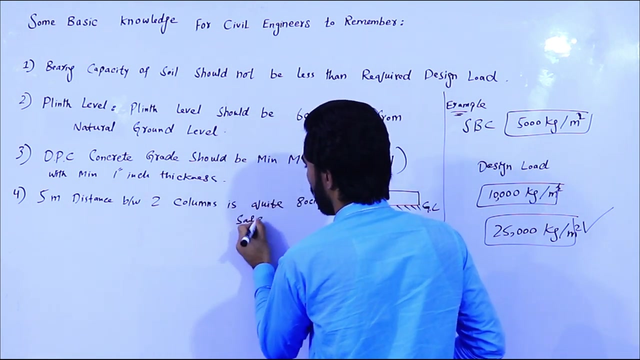 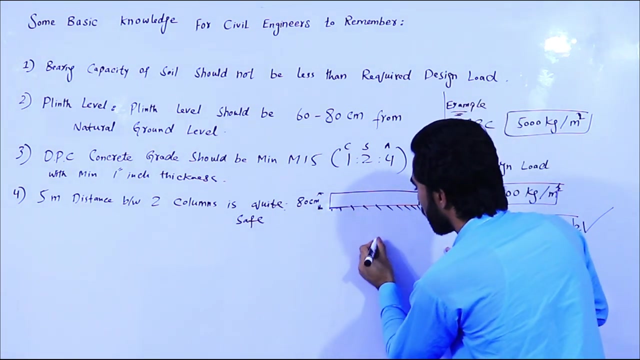 between two rcc column. but five meters, remember, five meter distance between two columns is quite safe. okay, five meter distance between two column is quite safe, so you can keep the distance between two columns. sorry, this is one column and this is other column, right? so, guys, the five meter distance is quite safe, but if you want to increase the distance, 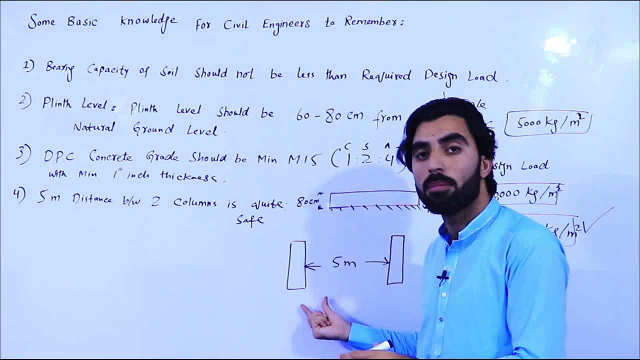 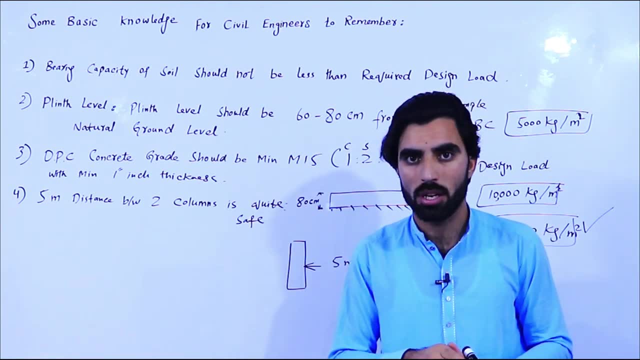 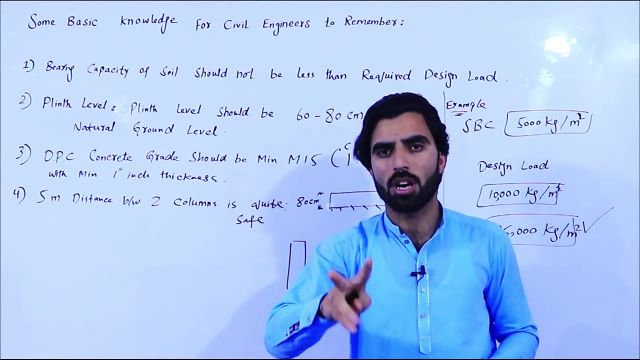 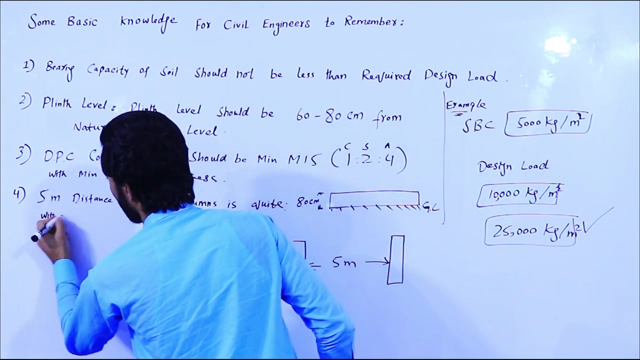 between two columns. so you will increase the size of the column, the size of the beam, also the thickness of the slab, etc. so it's depend on the structural design. but up to five meter distance between two rcc column is quite safe. but remember, guys, the grade width with minimum m20 grade concrete minimum with: 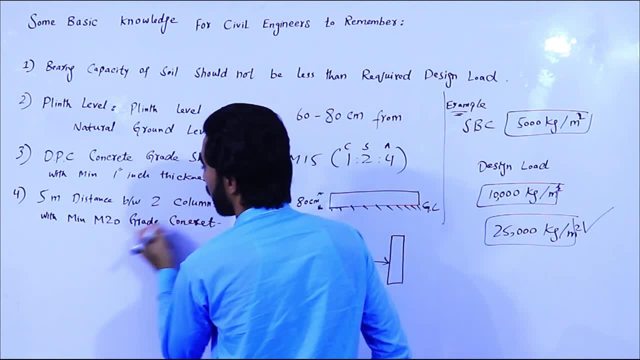 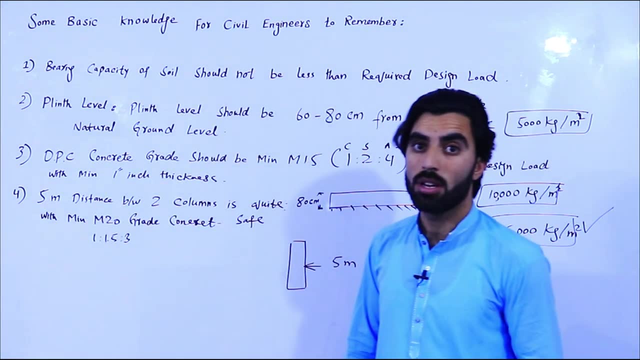 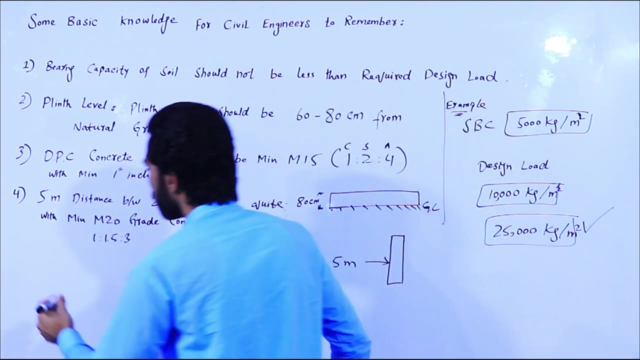 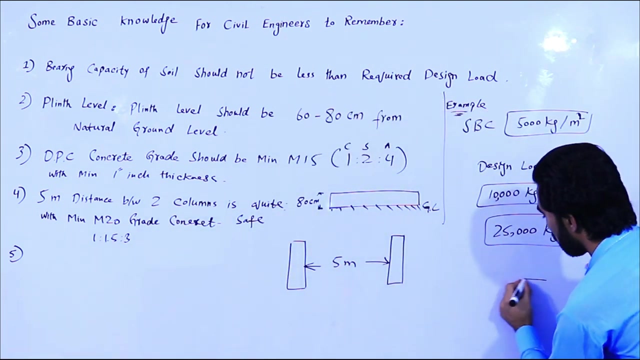 m20 grade concrete. where the ratio of m20 grade concrete is 1: 1.53, where one is cement, 1.5 is カル polished and like 2 degree on average across four sides, like mesh styrene. one will and 3 s crush are sacred, because this is the other point. 5th, guys, this is related with 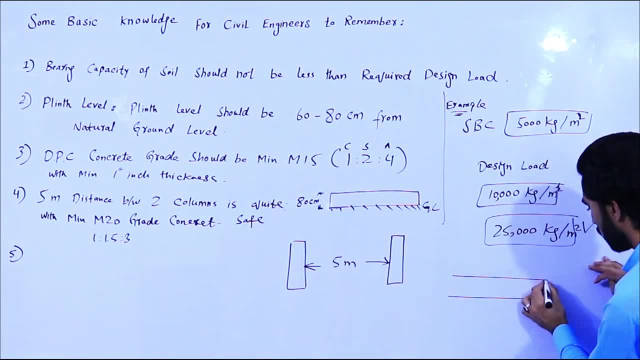 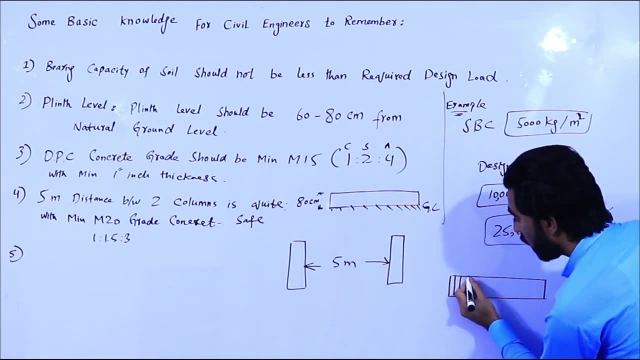 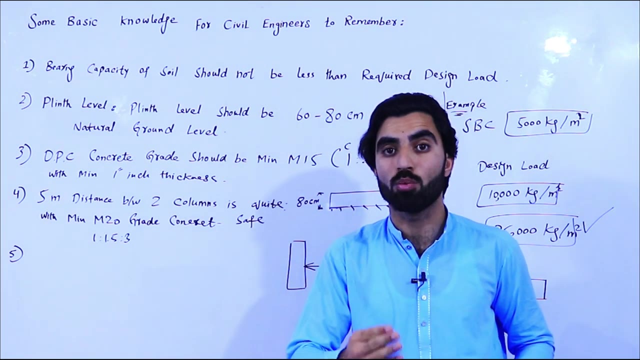 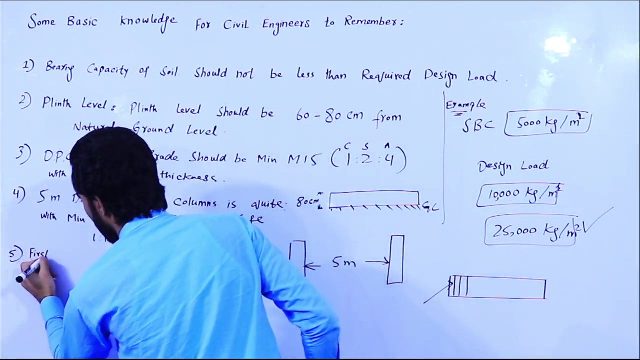 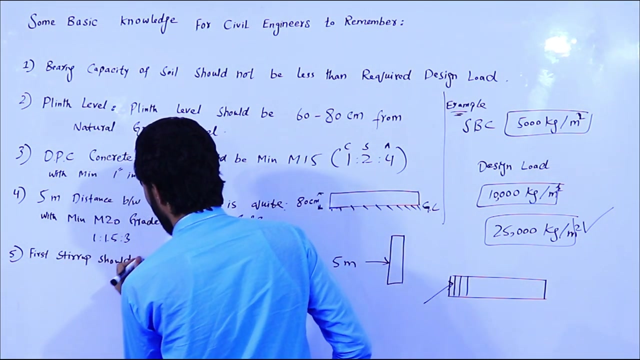 be. as you can see, guys, this is the beam long section about related with stirrup. guys, here, the 1st air of the first one stirrup, the first one in 3, is the motor느 cam. first stirrup and beam should be placed with minimum 2 inch distance. ok, first stirrup should. be placed minimum with 2 inch distance. so other edge depend on the structural design and it's also depend on the shear stresses etc. but the first, also from each side. the first stirrup should be placed minimum with 2 inches, the other one if there is. 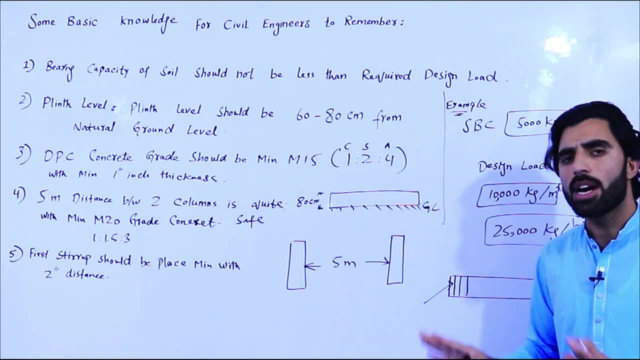 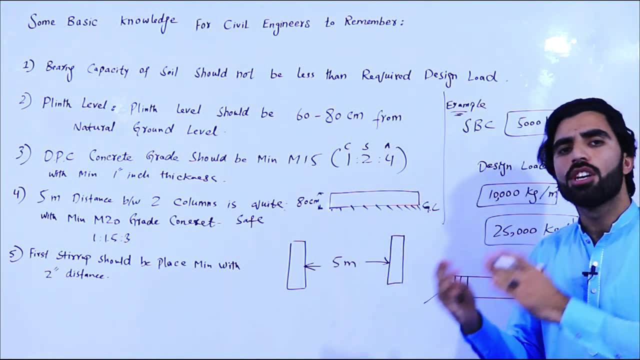 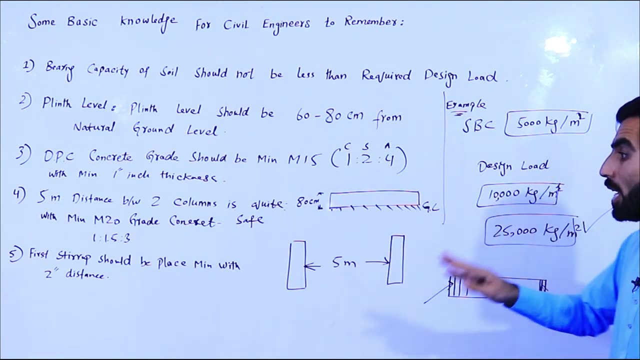 the limit, for example, if there is 4 inch, 6 inch or 7 inches, 7 inch. so I don't want to say something new in this because it is depend on the shear stresses. also it's depend on the structure load etc. structural design. but the first one stirrup should be placed minimum with the 2. 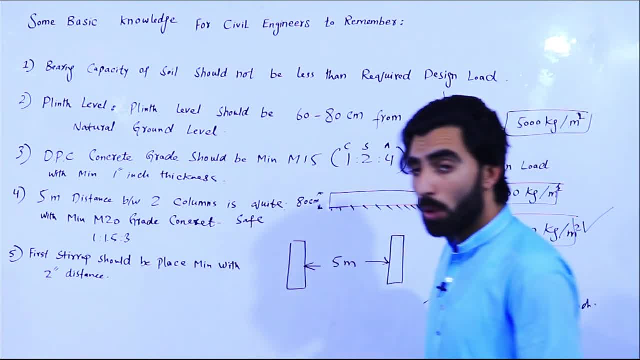 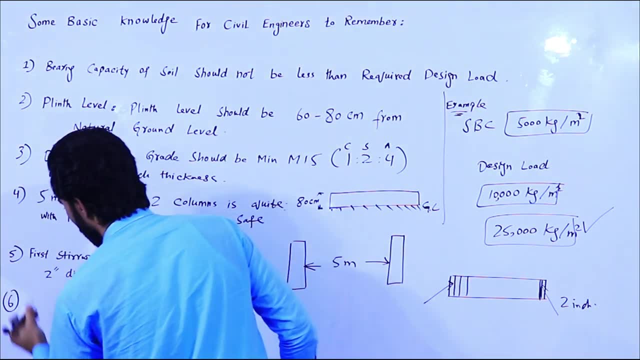 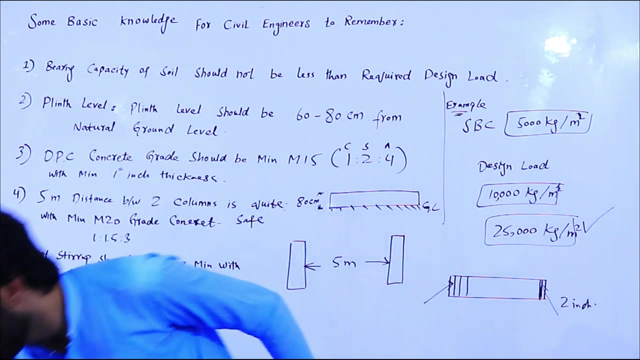 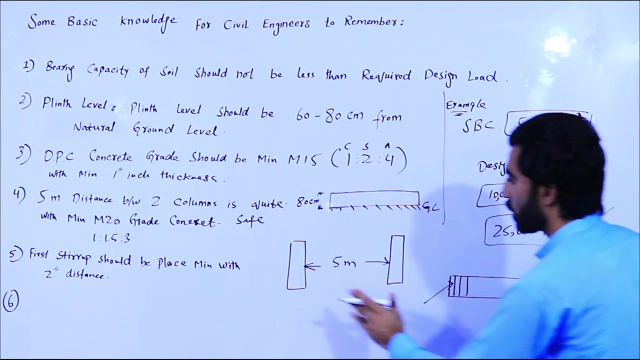 inch distance. this is the other point now, guys, in basic knowledge. the sixth one is also: okay, guys, this is also related with, and so I have yes, about development length. okay so, guys, and beam development length. here, guys, you can see, I will erase this. okay so, guys, you can see. 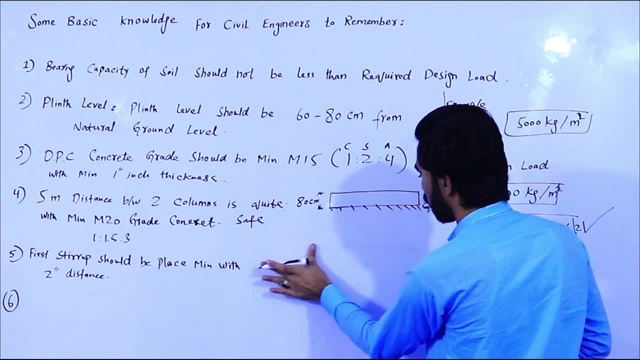 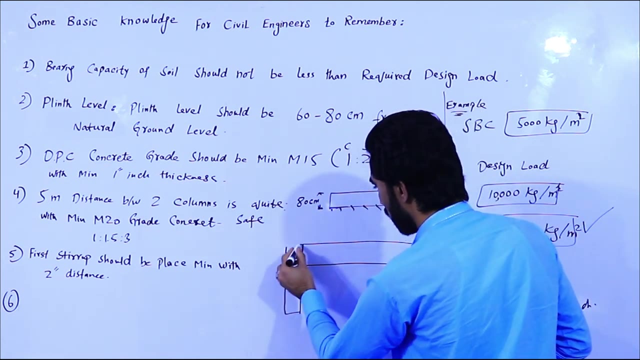 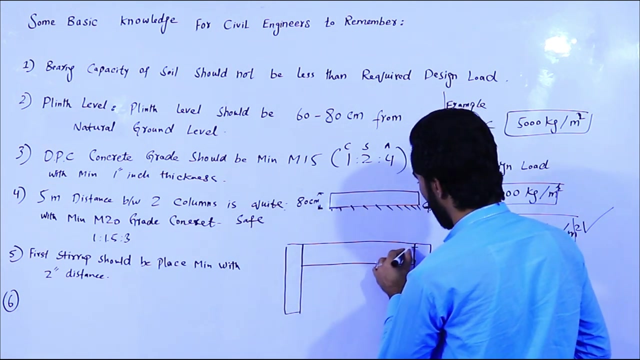 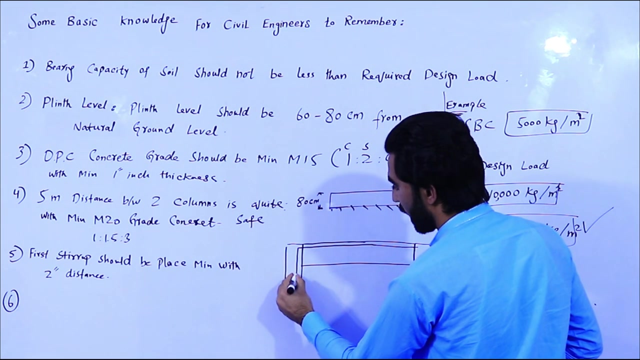 here. this is the long section of the beam beam long section. okay, so, guys, we have here also here, this is one column and this is other column. right, guys, here we have the steel bars like this. okay, so, guys, you can see this is the steel bar. here the steel is bent to the downside. guys, 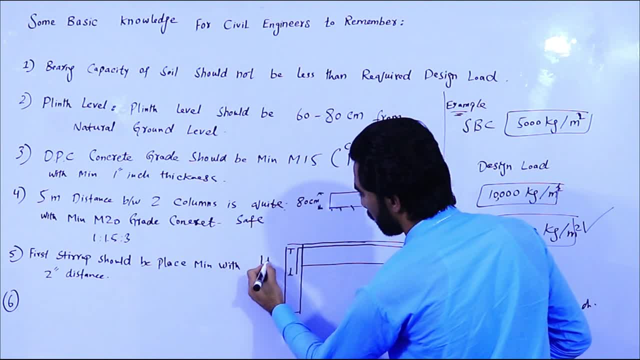 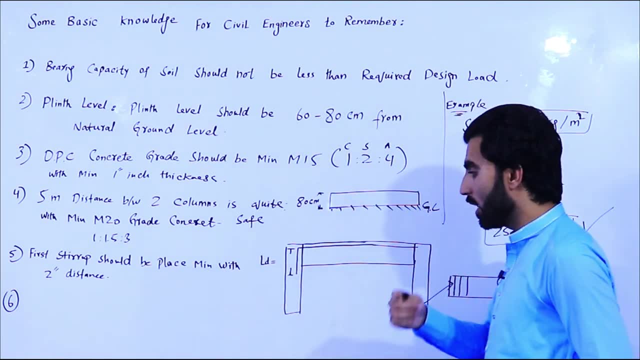 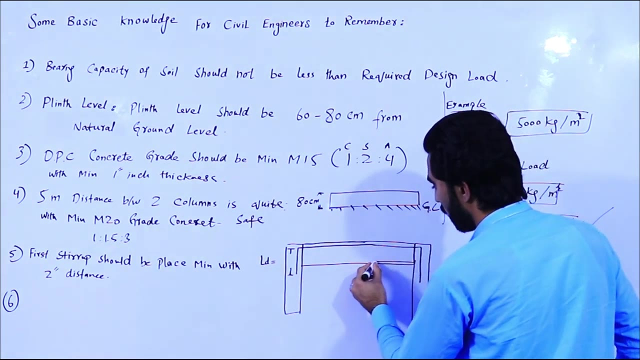 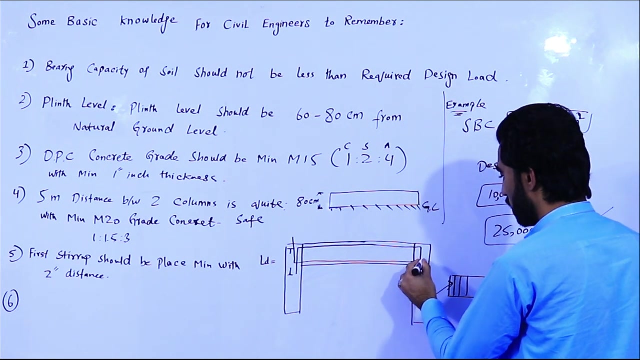 development length. this is called ld. this is development. so what should be the length of minimum length of development length? okay, development length, and also this one will be going to the also downside, and here this steel bar should be going to the upward side. this is the okay. so what should be the length of development? okay, so what should be?